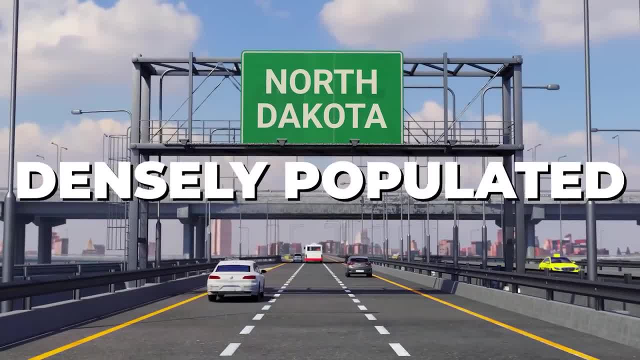 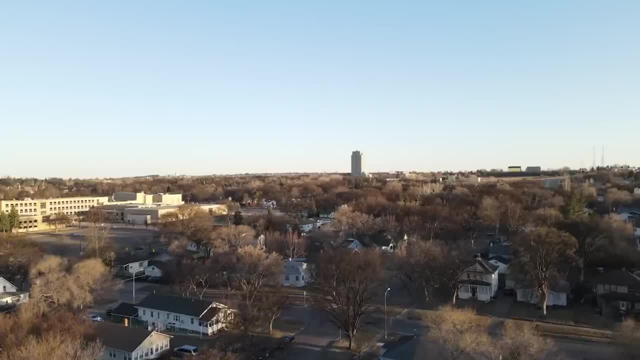 Did you know that North Dakota is the fourth least densely populated state in the whole country? While it has some beautiful national parks, a growing job market and a pretty low cost of living, there are some less obvious signs why this state is home to so few Today. 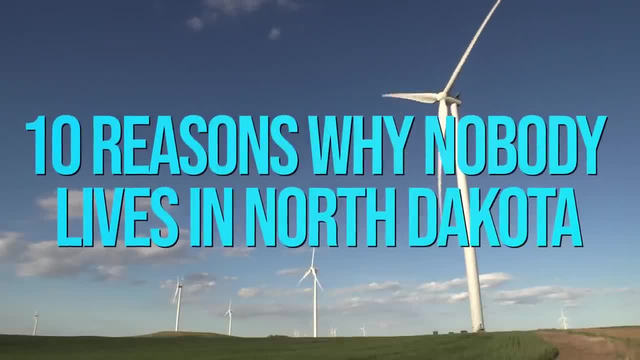 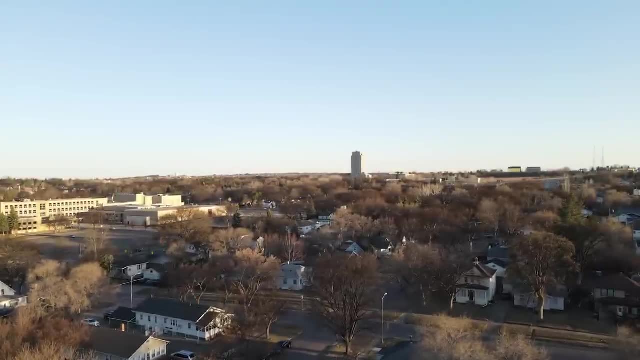 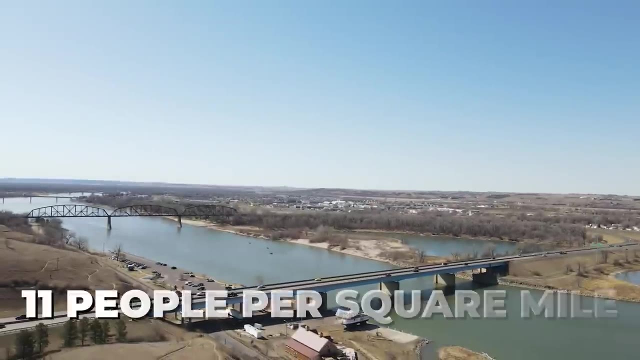 on Across the Globe. we're looking at the 10 reasons why nobody lives in North Dakota. 1. It's Boring. As I mentioned, North Dakota is the fourth least densely populated state in the entire country, For some perspective. it has around 11 people per square mile and a total population of about 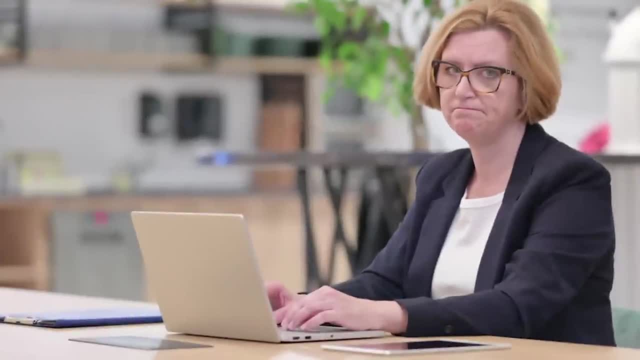 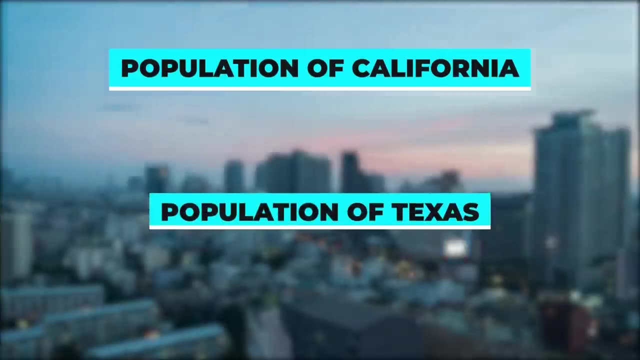 778,000.. You heard that right. the entire state is less than a million people. For reference, the most populated states, California and Texas, have populations of about 39 million and more than the rest of the United States. However, North Dakota is the fourth least densely. 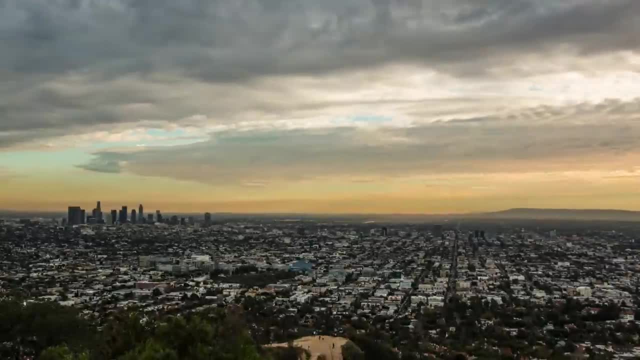 populated state in the entire country. For reference, the most populated states, California and Texas, have populations of about 39 million and more than the rest of the United States. In other words, California is 50 times the size of North Dakota and Texas is 37 times the size. 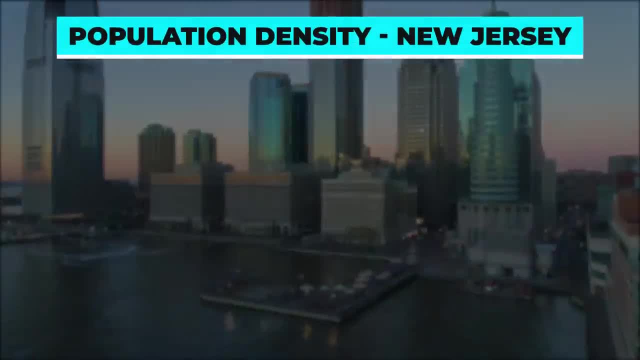 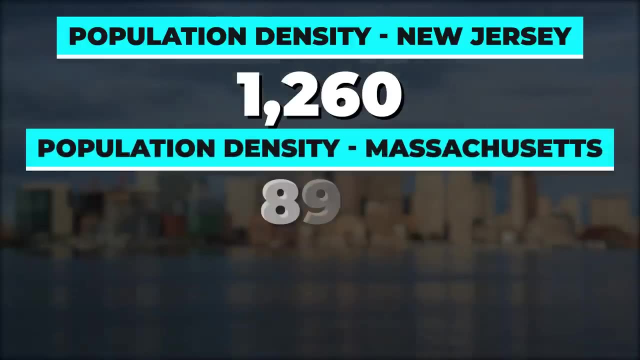 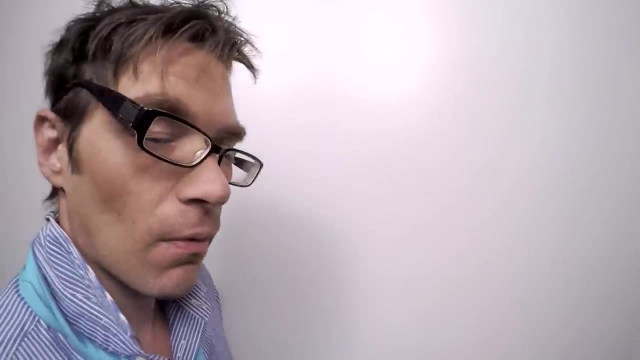 And in terms of population density, states such as New Jersey, for example, have a population density of about 1260, and Massachusetts is about 895,, which makes North Dakota's 11 seem almost unimaginable. With little to do, you might even develop a drinking problem, Unfortunately. I'm not kidding. A recent study found that North Dakota ranked highest for binge drinking, with an estimated 24.7% of adults reporting that they binge drink or drink heavily. This unfortunately also leads to a high number of DUIs and alcohol-related accidents, as the study found. 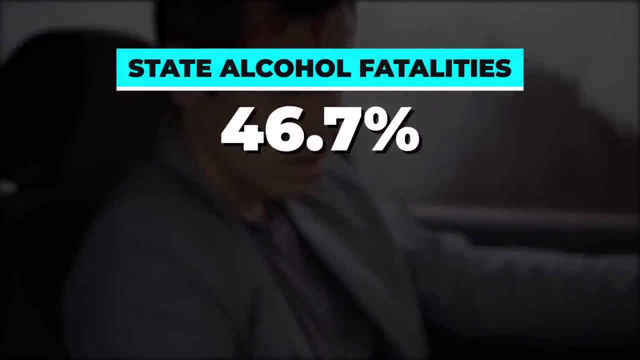 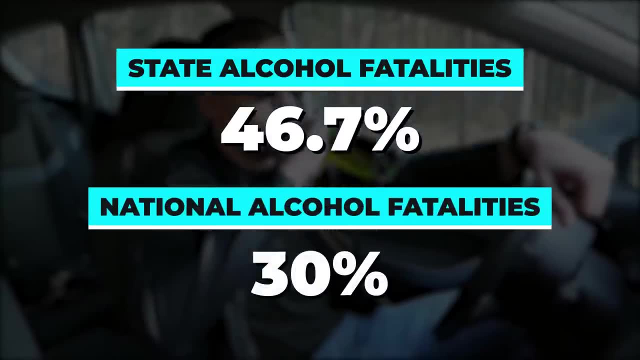 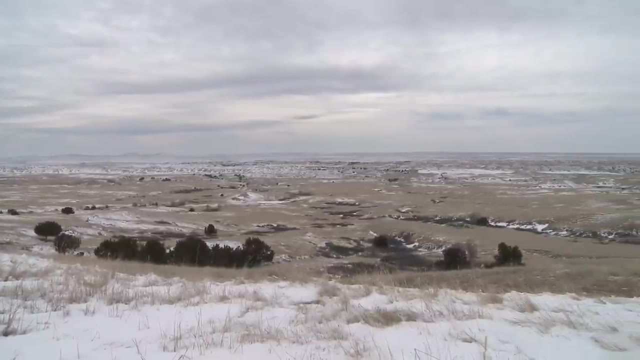 that in North Dakota, 46.7% of all roadway fatalities were due to alcohol consumption, far above the national rate of 30%. 2. It's freezing. If you ever visit North Dakota, you may experience being the coldest you've ever been in your life- Sub-zero temperatures. here are made. 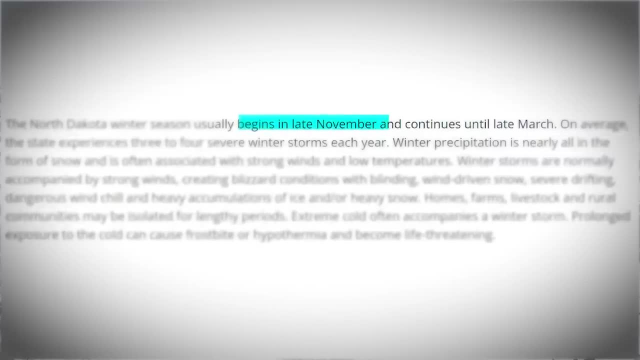 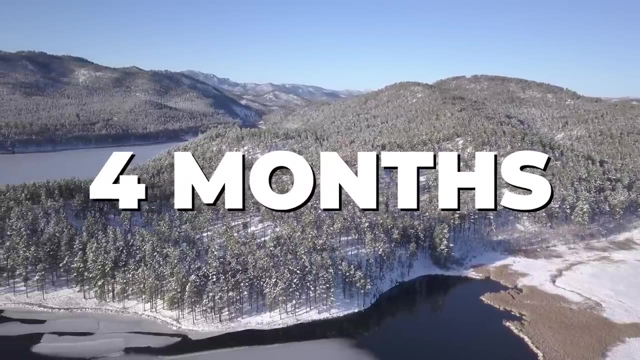 worse by a freezing wind chill. North Dakota winter usually begins in late November and continues through March. I'll do the math for you: That's four months of winter, or winter for over 30% of the year. If that still doesn't sound that bad to you, consider: 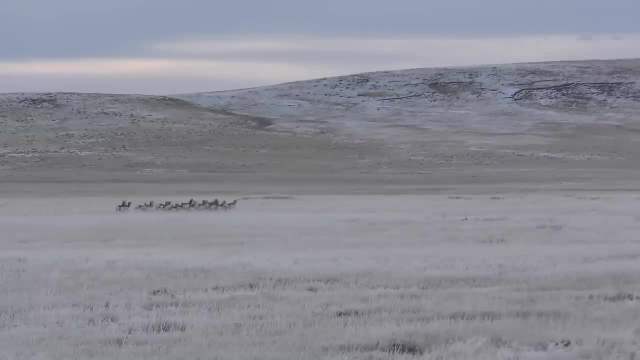 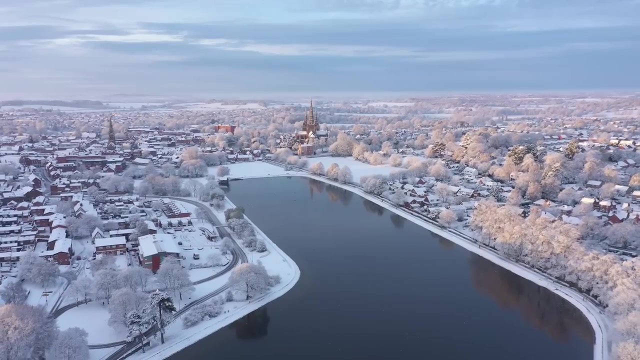 this: The average annual temperature in southern North Dakota is 43 degrees Fahrenheit and northern Dakota is 37 degrees Fahrenheit. That's the average year-round, including in the summer. So if you're looking for 80-degree summer days where you can jump in, 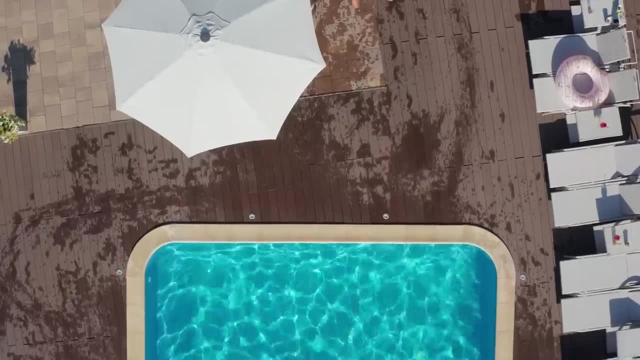 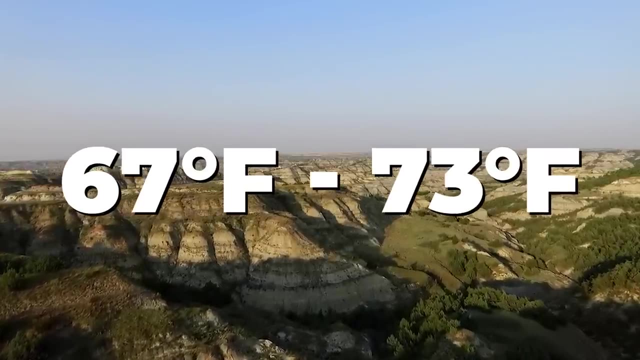 the pool. you're going to be hard-pressed to find that July, for instance, is the warmest month in North Dakota, but that only means temperatures between 67 and 73 degrees. But what's worse are the winter averages. The average winter temperature in the south is: 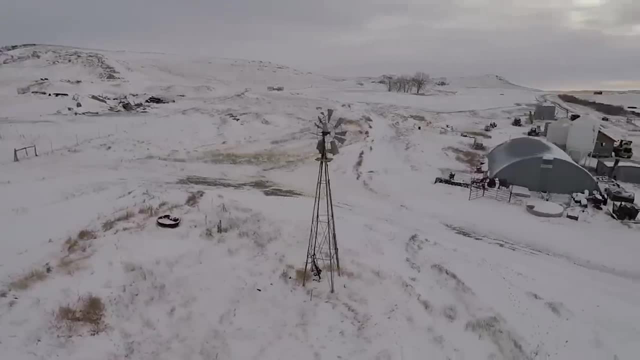 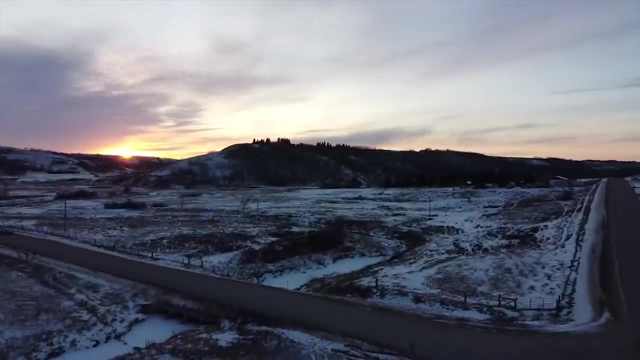 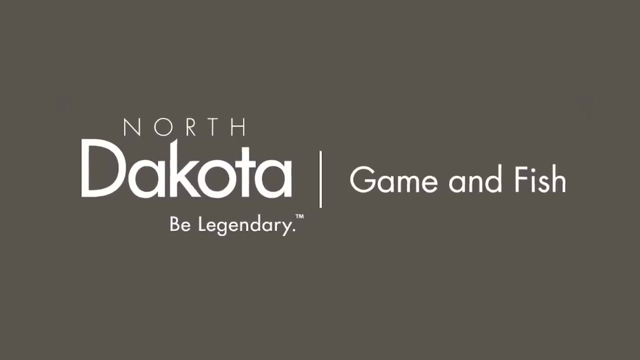 only 17 degrees Fahrenheit and in the north only 2 degrees. In case you didn't hear that, I'm going to repeat it: 2 degrees. Remember that these are averages, which means that North Dakota is seeing plenty of days below zero. How many days? Well, according to the North Dakota Game and Fish Department, 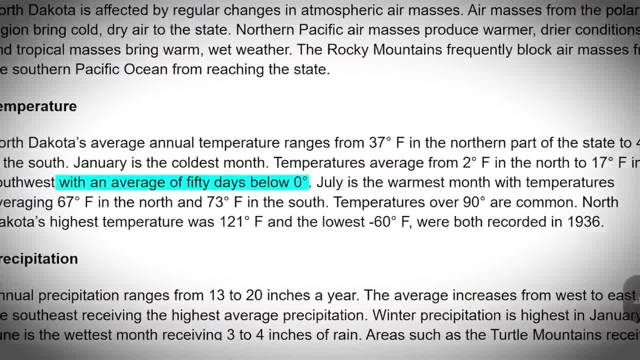 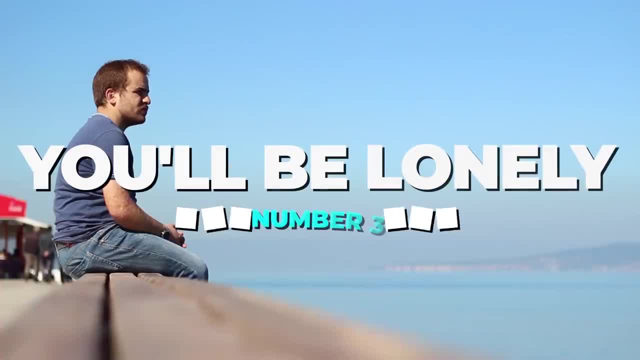 the state generally sees fifty days below zero. That's almost 15% of the average year-round winter. you're seeing in North Dakota, If percent of your days spent totally freezing, Number three- you'll be lonely. As I've mentioned, North Dakota has a tiny population, at least relative to other states. 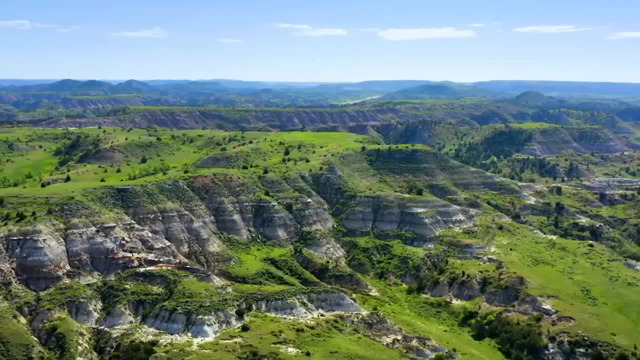 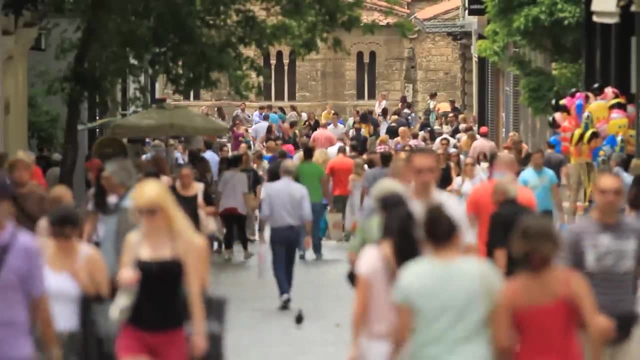 But a tiny population doesn't necessarily mean you'll be lonely. After all, if most of the population was located in one big, friendly, fun city, you'd be sure to meet tons of people and make lots of friends. Unfortunately, that's not really the case here. 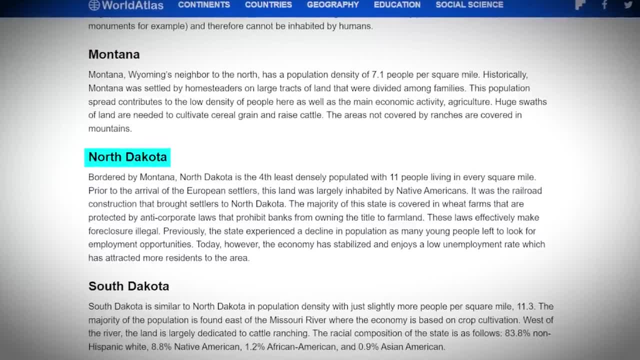 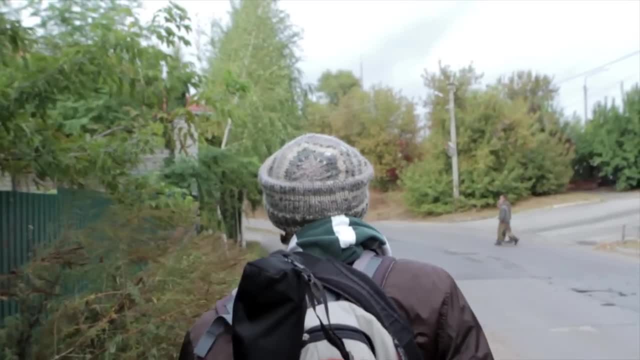 In fact, according to World Atlas, North Dakota is the fourth least densely populated state in the entire country, as it has only about 11 people per square mile. That means if you were to walk one square mile, you'd only encounter 11 people along. 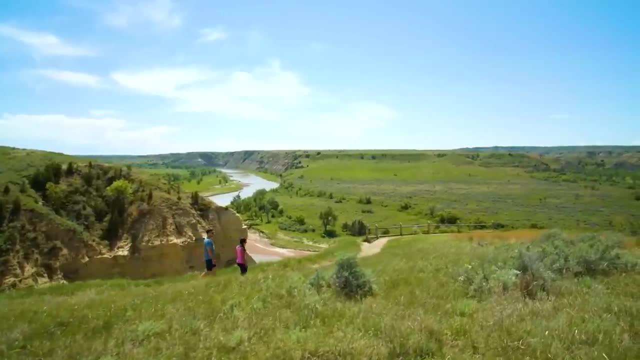 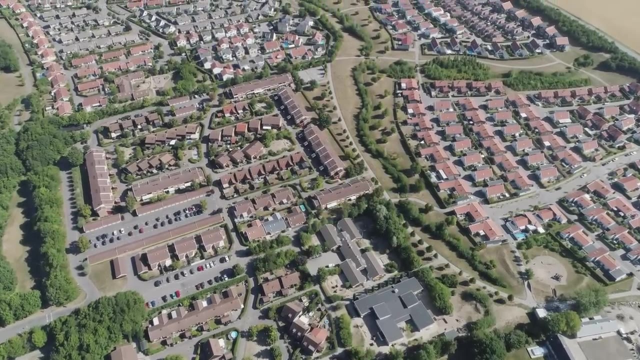 the way. What this means is that most of the state is pretty rural. Miles can stretch between houses And if you're picturing a nice neighborhood vibe, you're probably going to need to look elsewhere. And while the people of North Dakota are generally considerate North Dakota is one of the most 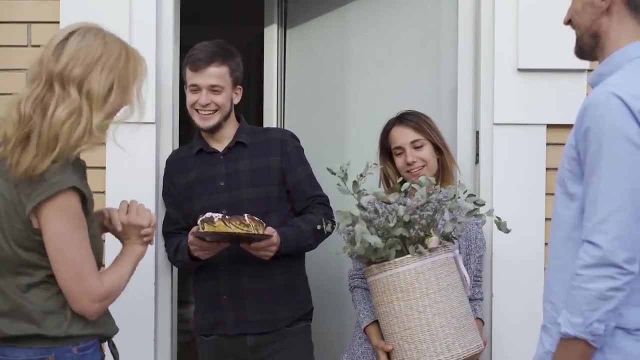 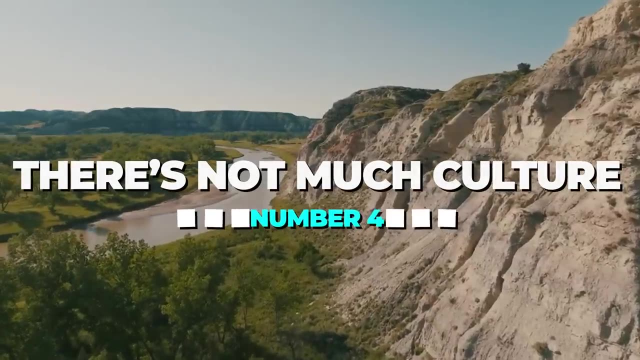 popular states. in the United States, It's considered to be friendly and welcoming towards strangers. That doesn't really matter a whole lot if you don't encounter them on a day-to-day basis. 4. There's Not Much Culture. There's also not a ton going on in terms 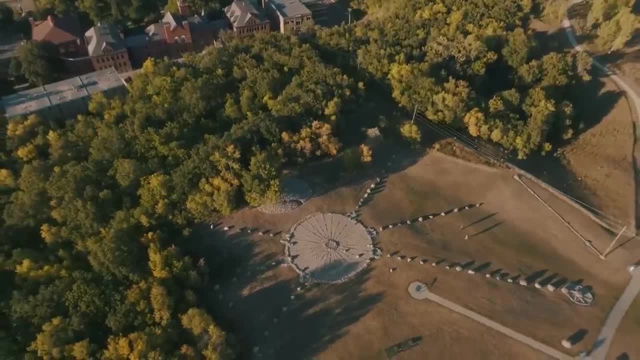 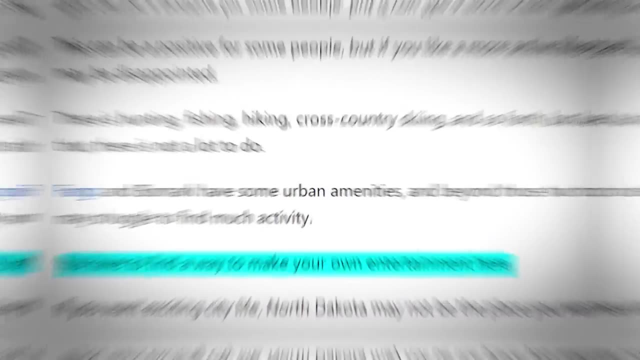 of culture. here. The arts and entertainment scene is pretty lacking. In fact, most travel blogs that we looked at mentioned how little North Dakota has in terms of entertainment If you're looking to go out to museums every once in a while or see an up-and-coming band. 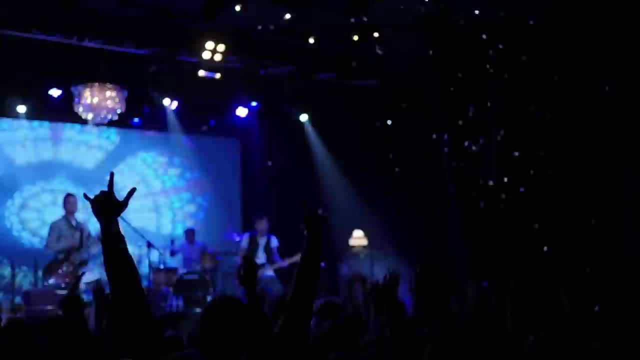 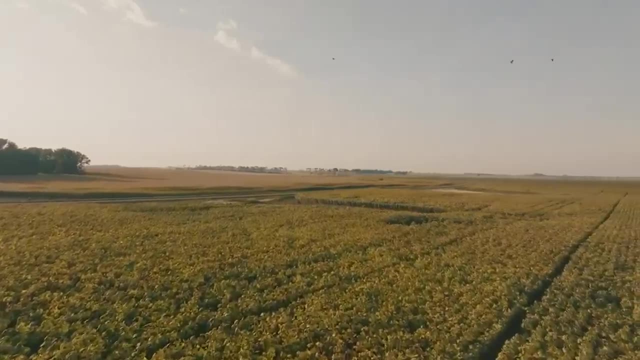 or play in a cool venue, you probably won't have much luck and may even need to travel out of state to get that. Yes, there are some museums and live shows here, but not many. So if you live here, you'll probably have seen all North Dakota has to offer arts-wise. 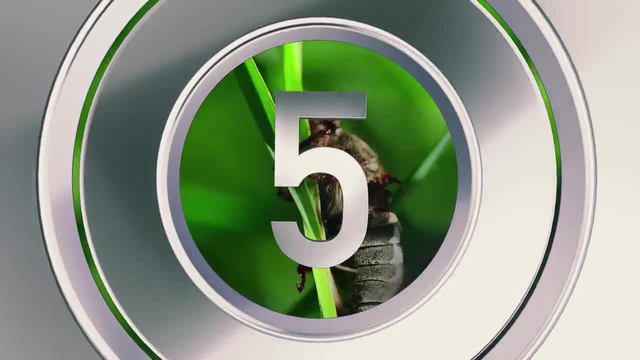 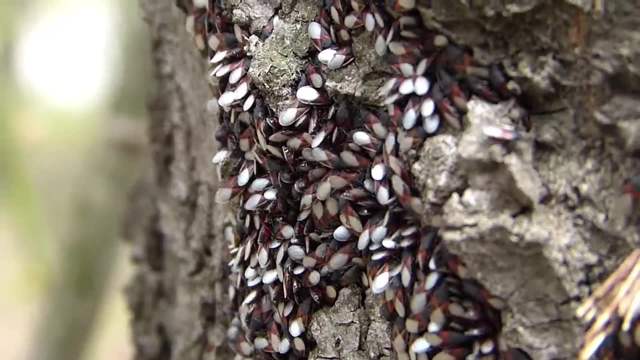 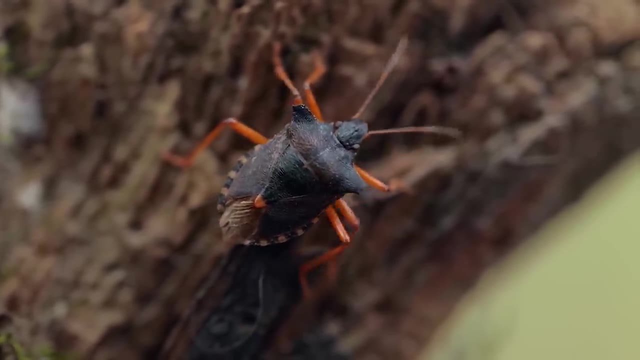 within just a few short months. 5. The Bugs: I know you're probably thinking that bugs are everywhere. Can it really be that much worse in North Dakota? It can. 5. The Bugs here are so creepy that they'll creep out even the bug lovers among you. 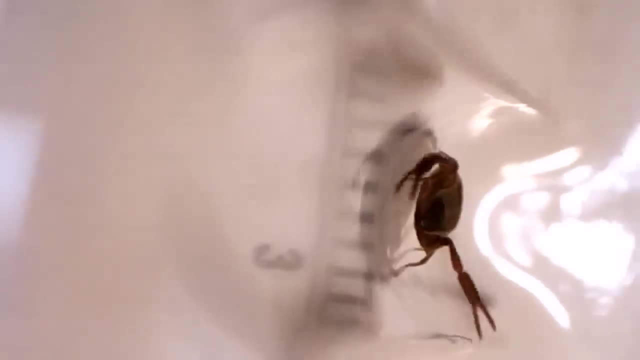 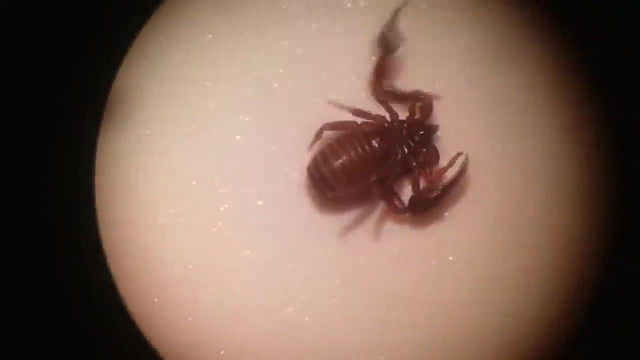 Let's start with Pseudoscorpion. Yep, it's a bug that looks like a scorpion. North Dakota isn't remotely close to the desert, but somehow this little guy made its way across prairies and fields to settle down in the houses of North Dakotans everywhere. 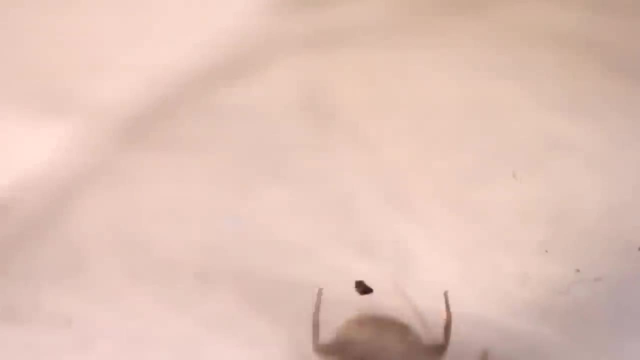 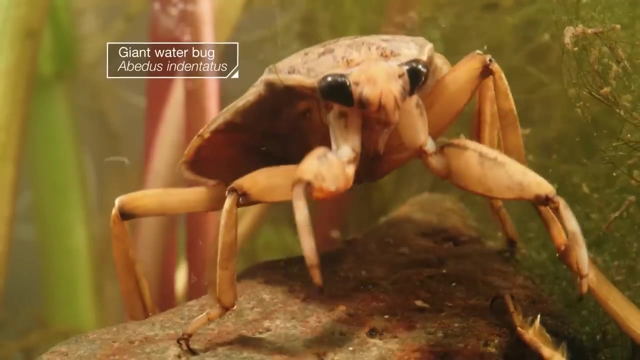 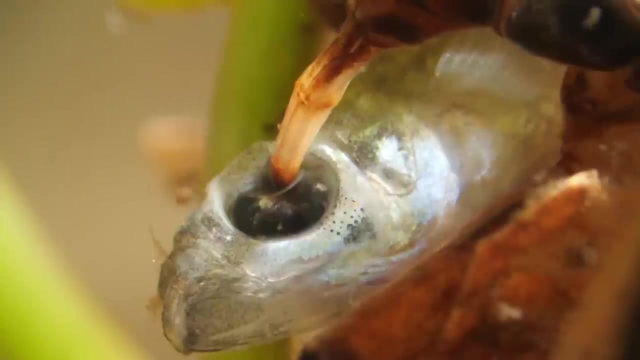 While the bug is usually not deadly, it is creepy and definitely not something you want to find scurrying around your house. Then there's the giant water bug. These can get as big as four and a half inches long. Found in bodies of water, they hunt and eat small fish, frogs and other bugs. 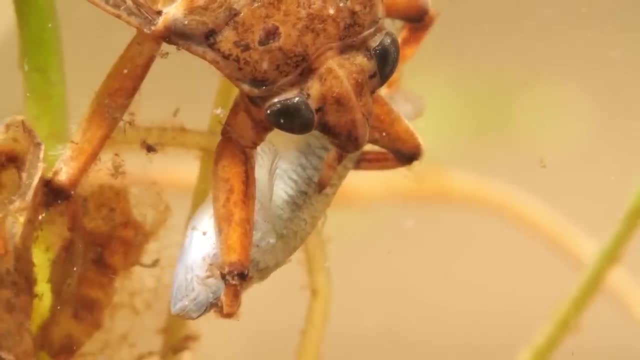 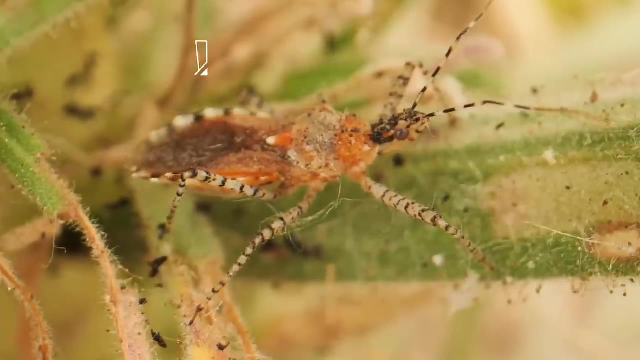 So even if you found a crystal clear freshwater pond that looked like a great place for a swim, it might be ruined by running into one of these creepy crawlers. But my personal favorite- and I'm saying that sarcastically- is what's known as the 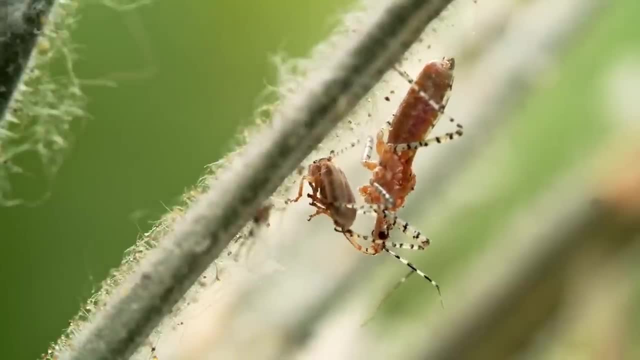 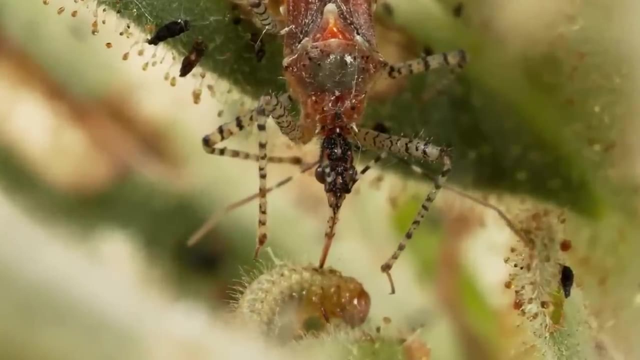 assassin bug. As if its name weren't bad enough, this bug can stab its prey, injecting a venomous so-called poison that is so painful that it might send you racing off to the hospital Number 6.. There are housing problems. 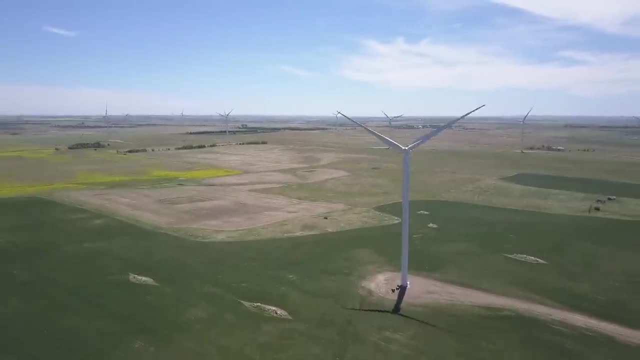 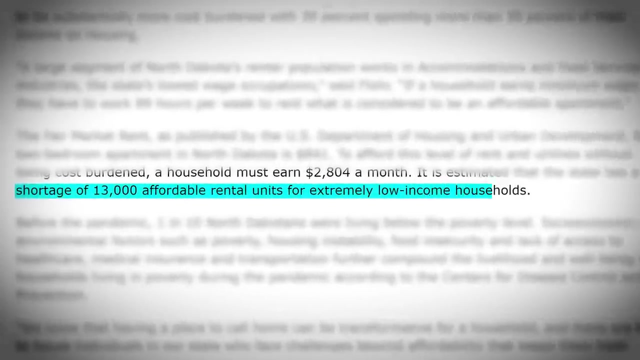 You might think that, in a state with tons of open land, that there would be plenty of available housing options, but that's actually not the case. It's estimated that North Dakota has a shortage of 13,000 affordable rental units for low-income people. While 13,000 might not seem like a whole lot, remember that the entire population is only 778,000. And considering that 1 in 10 North Dakotans are living below the poverty level, that really is a problem. People are also spending a disproportionately high amount of their income on housing too. 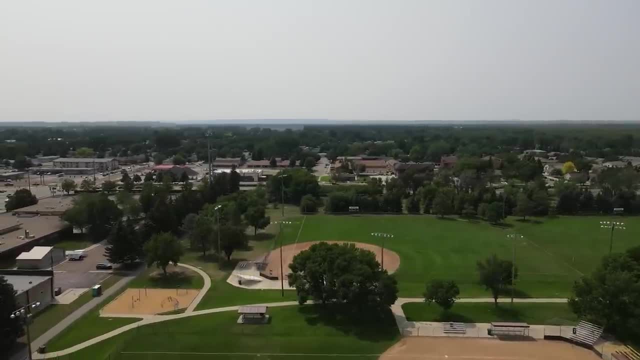 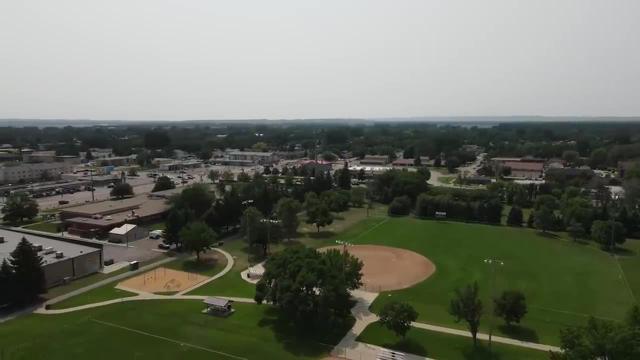 There's a general rule of thumb amongst financial advisors that you shouldn't spend more than 30% of your income on housing. yet in North Dakota, 39% of those who rent spend more than a third of what they make on housing costs. 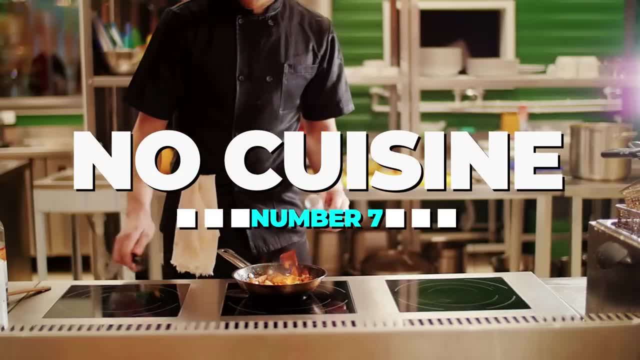 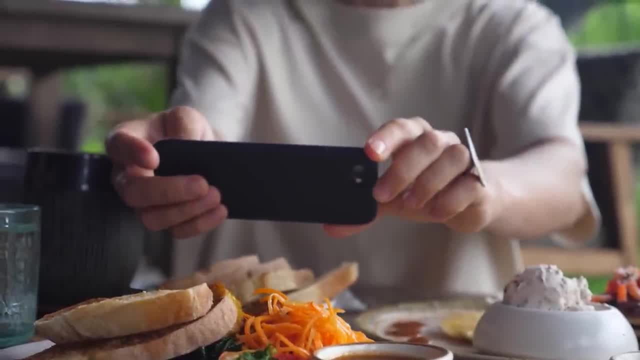 Number 7. There's no cuisine. North Dakota's food is notoriously bland. If you're a foodie looking to frequent the latest up-and-coming restaurants, or simply someone who likes trying out different cuisines, you won't find much of that here. 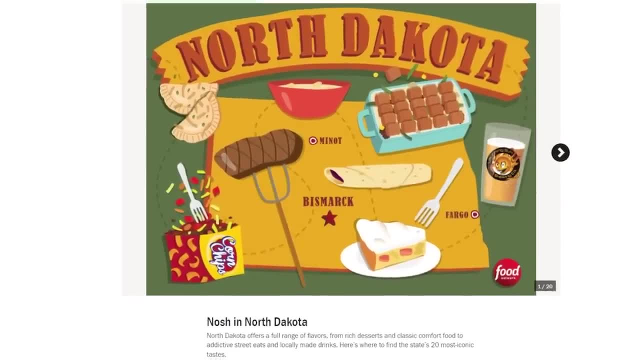 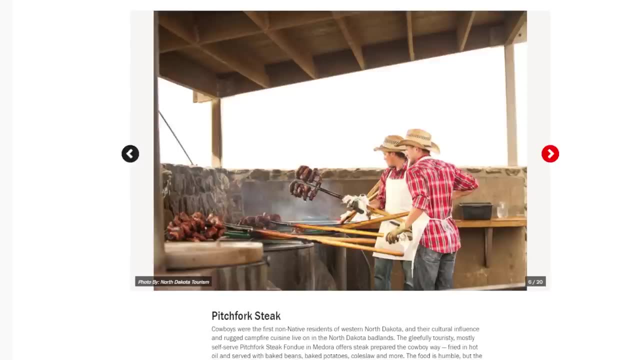 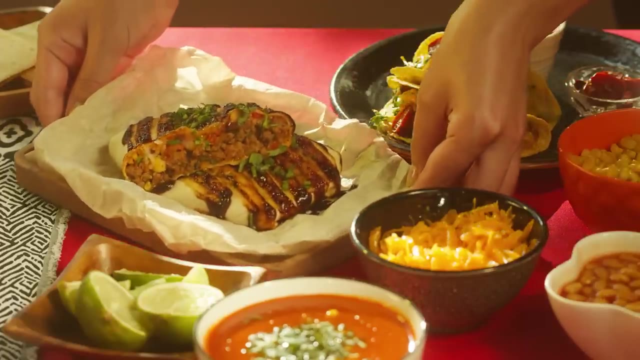 The Food Network recently listed some of North Dakota's culinary specialties and they looked pretty bland. These included things like a casserole made out of tater tots and a salad made out of get this jello. If you're looking to hit up the latest great sushi or Mexican restaurant, you probably 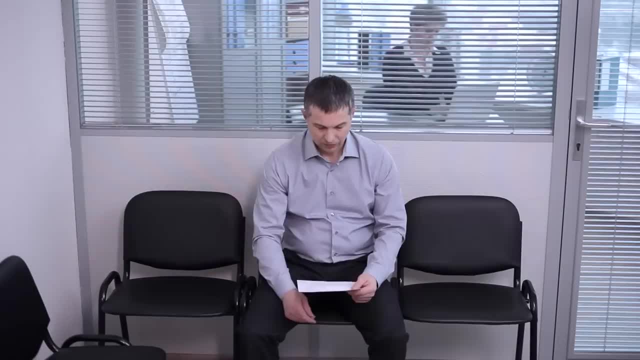 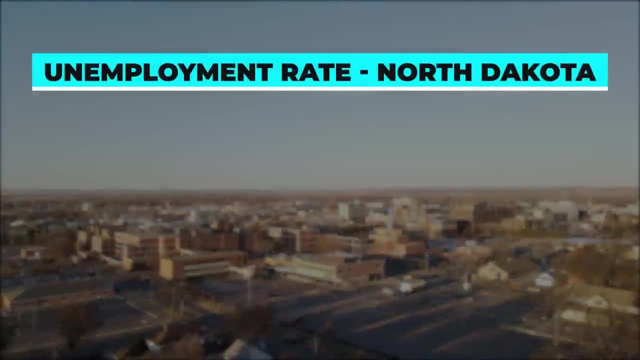 won't find it here, Number 8. There aren't many job options On paper. North Dakota has a pretty robust economy. As of November 2022, the unemployment rate was only 2.3%, which is well below the national. 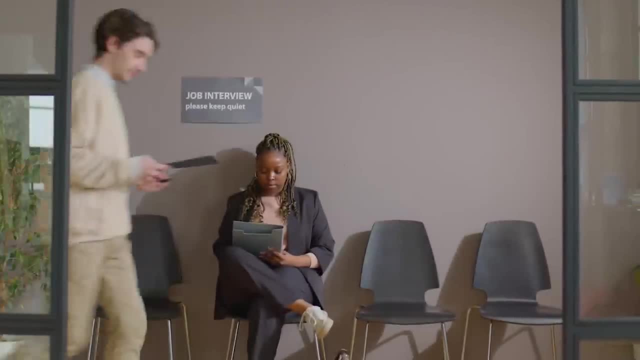 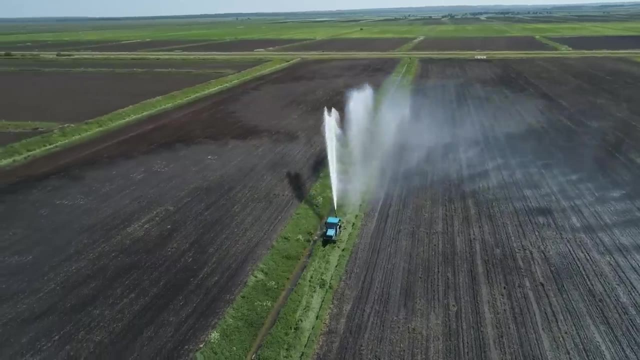 unemployment rate of 3.5%. But these numbers aren't all they're cut out to be. If you're looking to secure a job in the industries of mining, you're probably looking for a job in the food industry, But if you work in a more creative field or are looking for a career, that's a bit more. 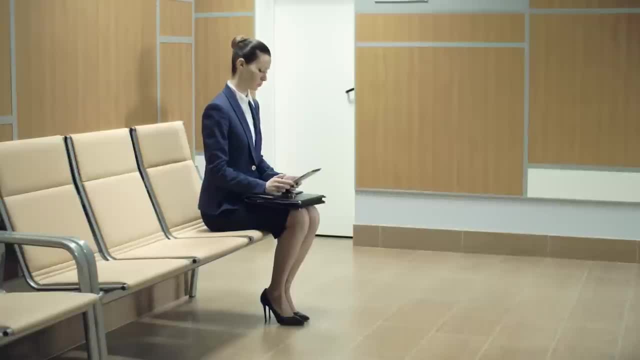 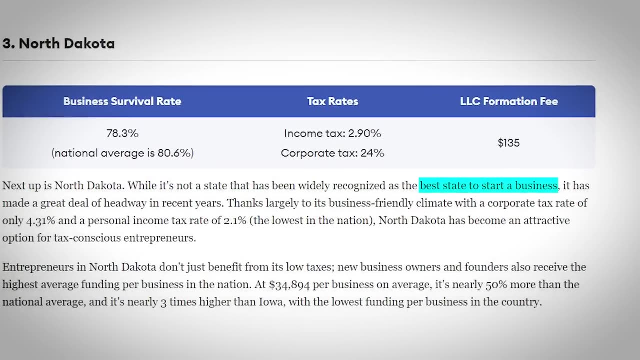 outside of the box, you'll have a harder time finding it here. Additionally, if you're a small business owner, you may have some trouble surviving. While the state of North Dakota is generally considered business-friendly, in recent years small businesses have struggled to find employees. 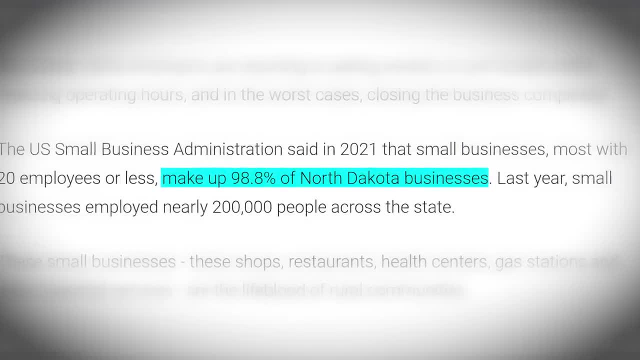 Considering that 98.8% of North Dakota businesses are considered small businesses. North Dakota's economy is not as good as it used to be. In recent years, small businesses have struggled to find employees. Considering that 98.8% of North Dakota businesses are considered small businesses, North Dakota's 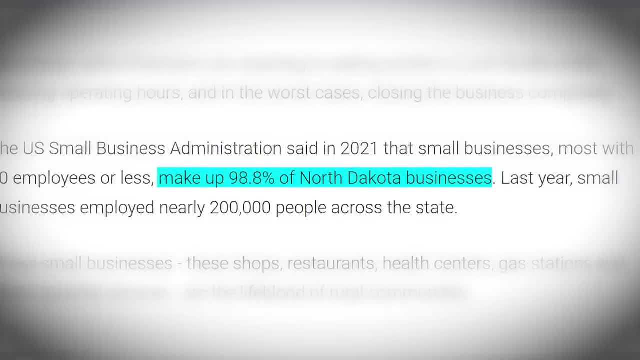 economy is not as good as it used to be. In recent years, small businesses have struggled to find employees. Considering that 98.8% of North Dakota businesses are considered small businesses, North Dakota's economy is not as good as it used to be. 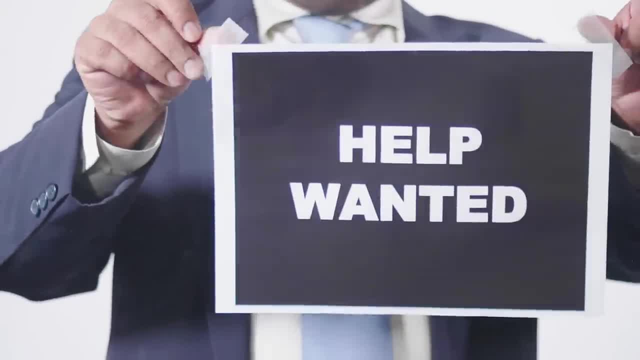 Considering that 98.8% of North Dakota businesses are considered small businesses, North Dakota's economy is not as good as it used to be In recent years. small businesses with 20 employees or less. this presents a huge problem. That's because being understaffed means that other employees are needing to work longer. hours or the business has to keep shorter hours. And as many rural communities in North Dakota rely on small businesses for food, gas and other essentials, this becomes an even bigger community-wide problem. 9. There's No Diversity If you're looking for a place with people. 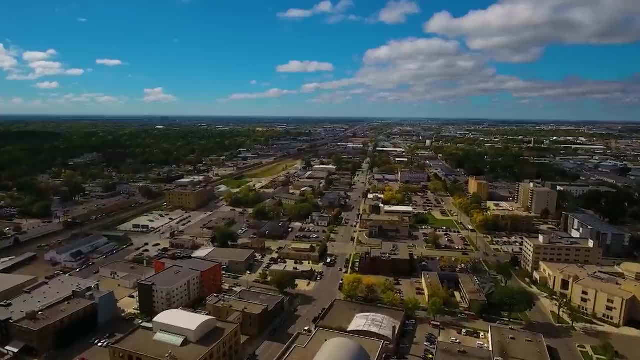 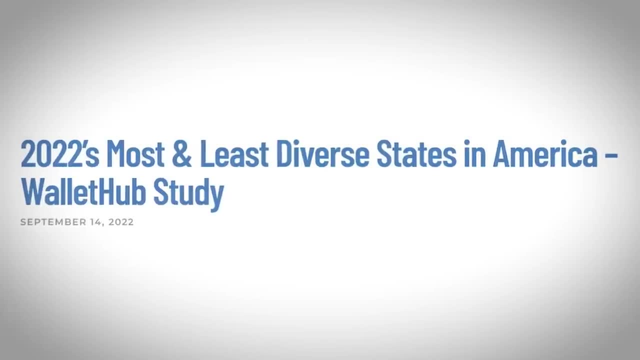 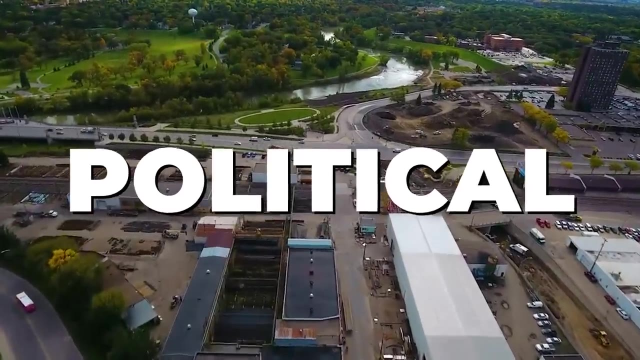 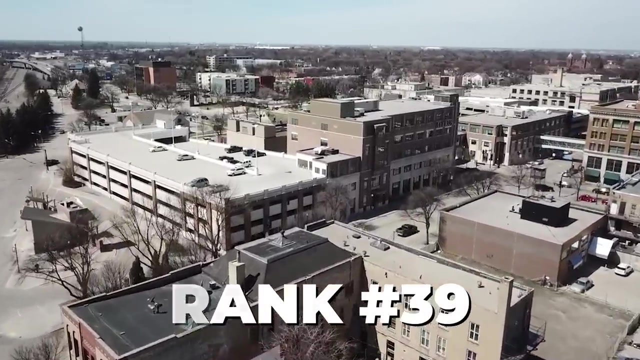 from different backgrounds with diverse options. you're not likely to find that in this state. WalletHub recently looked at states and compared their diversity levels across six diversity metrics—economic, socioeconomic, cultural, household, religious and political diversity. North Dakota ranked number 39,, making it one of the least diverse states in the country. 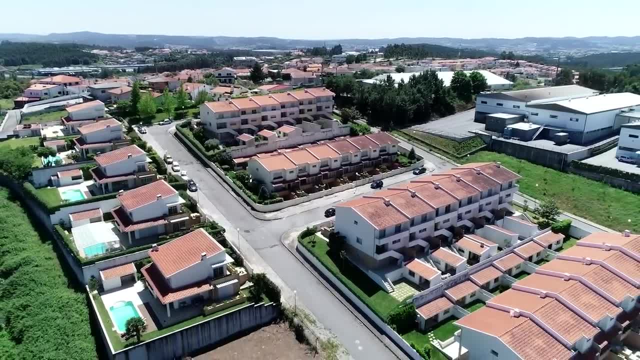 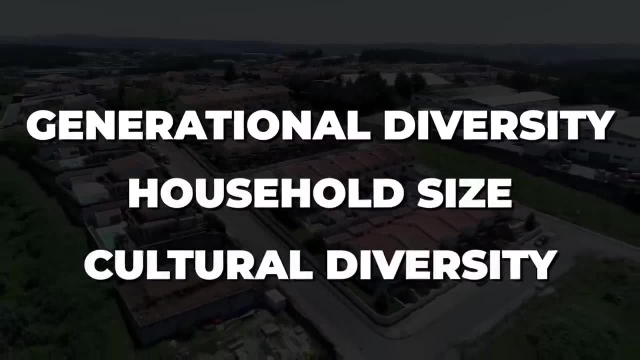 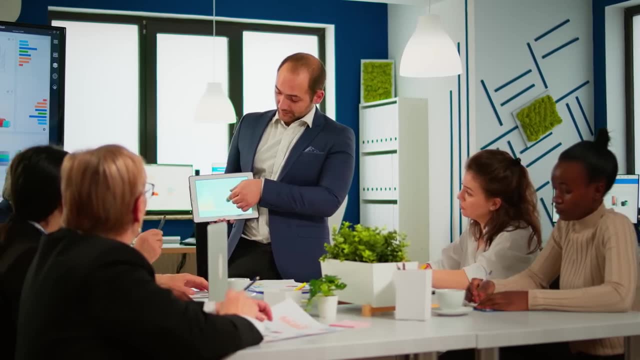 It ranked particularly poorly when it came to household diversity, which includes the factors like generational diversity and household size, and cultural diversity, which includes racial and ethnic diversity. Why is this so important? Well, studies have shown not only that people can benefit from diversity on an individual, 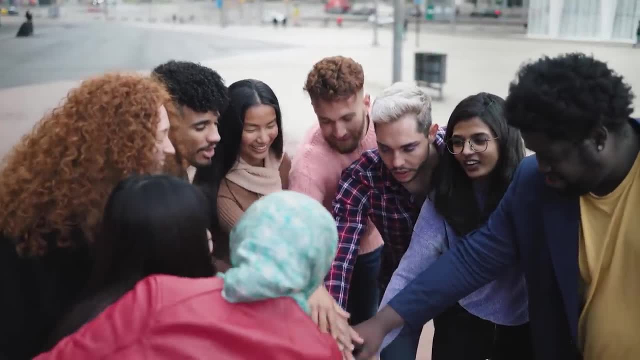 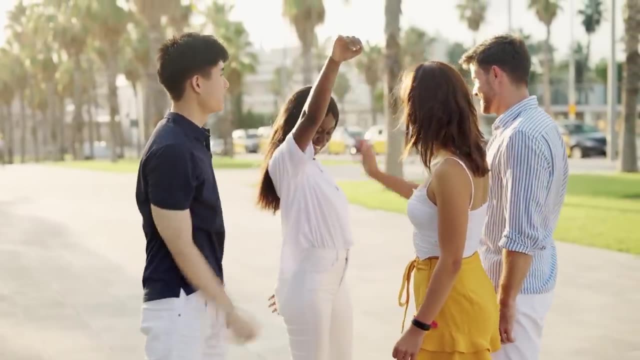 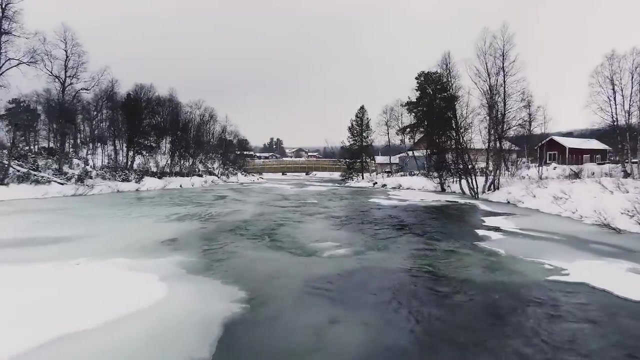 level, but that diverse workplaces and diverse schools outperform those that are less diverse. So, in other words, you won't be getting many of these benefits from living here. 10. There Are Tornadoes, As if sub-zero weather wasn't bad enough. people. 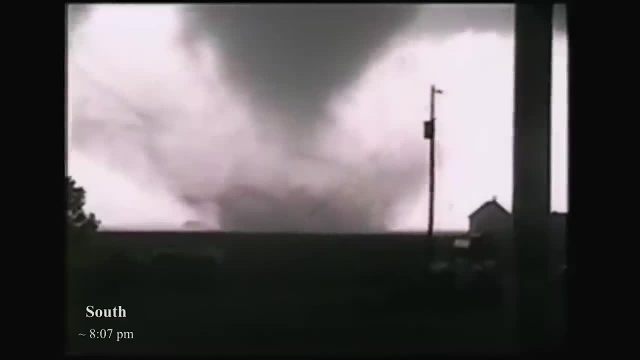 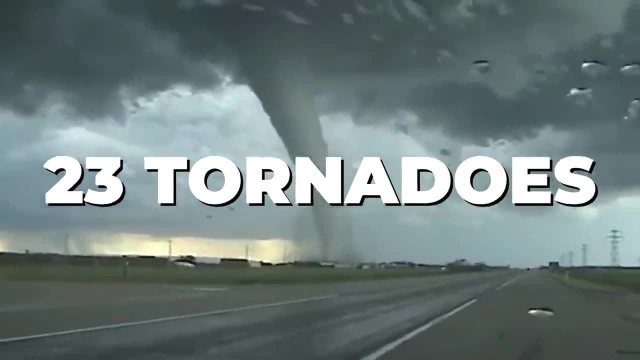 in North Dakota also have to look out for tornadoes, and tornadoes are a regular occurrence. In fact, North Dakota averages 23 tornadoes per year. That's almost equal to two tornadoes per month, and there's no relief from them either. 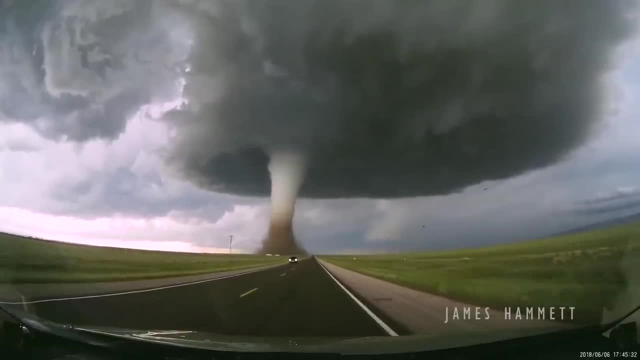 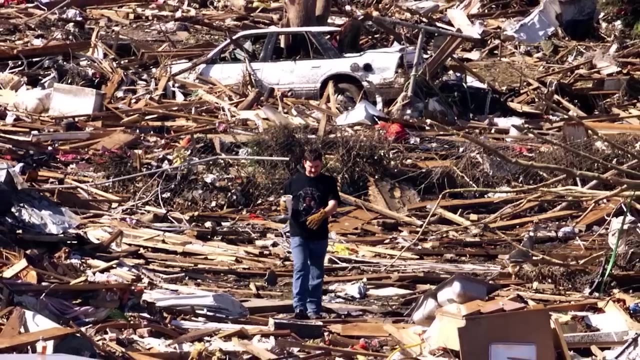 as tornadoes can strike at any time of year, at any moment. In other words, if you live here, tornadoes become a way of life 11. The Damage From Them Can Be Severe. A prime example of this is what happened after. 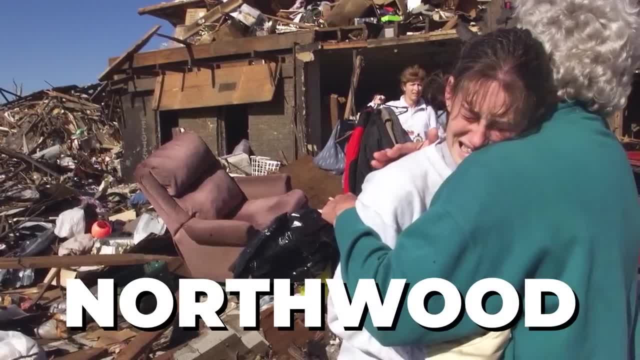 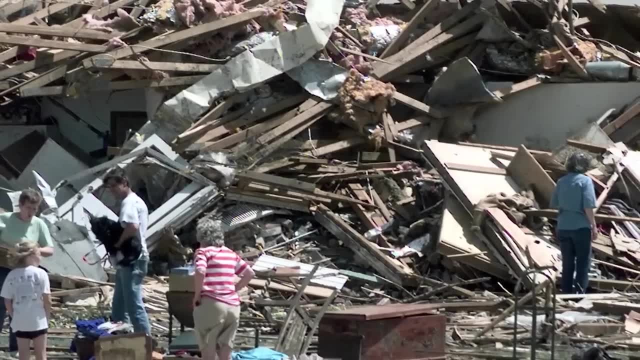 a tornado wreaked havoc on the North Dakota town of Northwood in August of 2007.. That led to one death and injuries to 18 other people. That may not seem like a lot, but considering the population of Northwood at the time was. 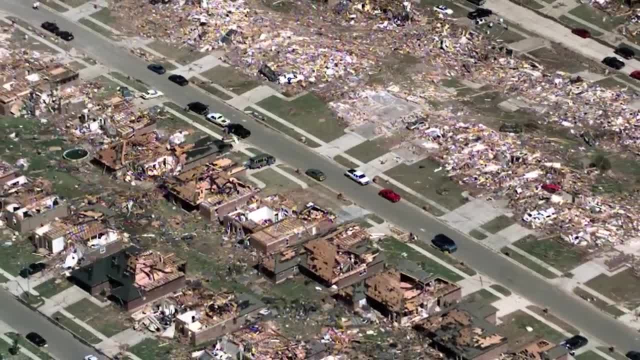 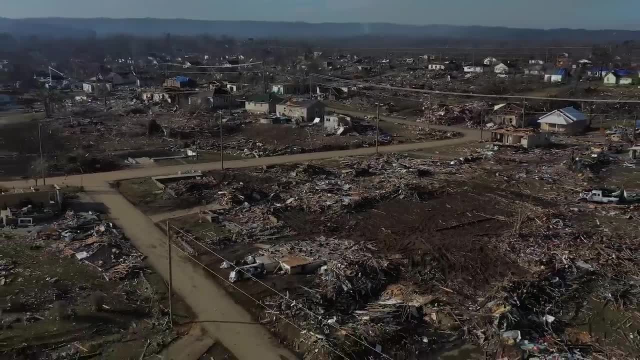 only 875 people, things become a bit more real. But the damage wasn't just physical, it was also financial. Data showed approximately 3.4 million people died in Northwood. That's a lot. That's 1.5 million in uninsured losses, as most homeowners did not have adequate insurance. 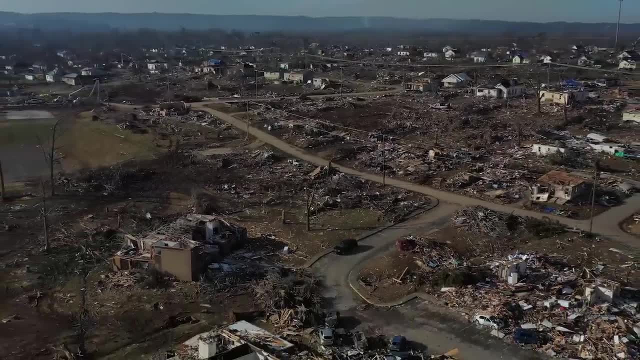 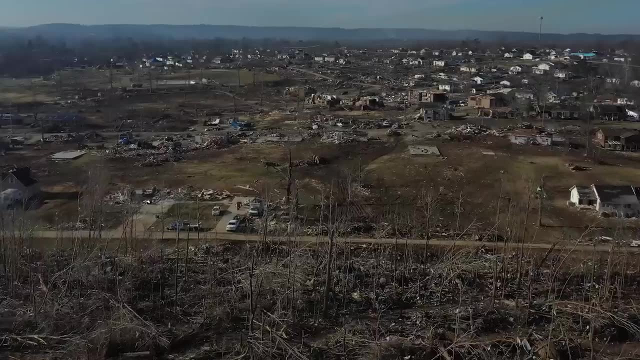 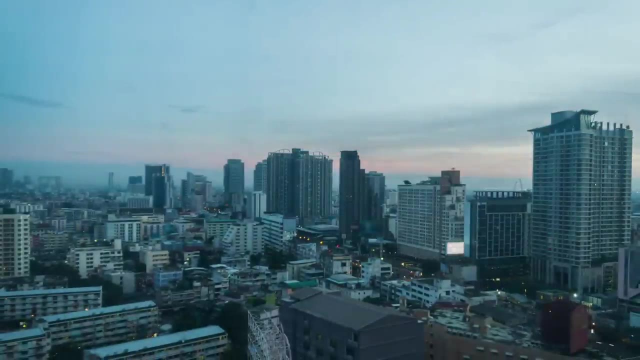 to compensate for the cost of rebuilding after the tornado. In other words, tornadoes here aren't just scary, they also create huge physical and financial damage to communities. What about the 10 cities everyone is leaving in America? Watch this video to learn about that.